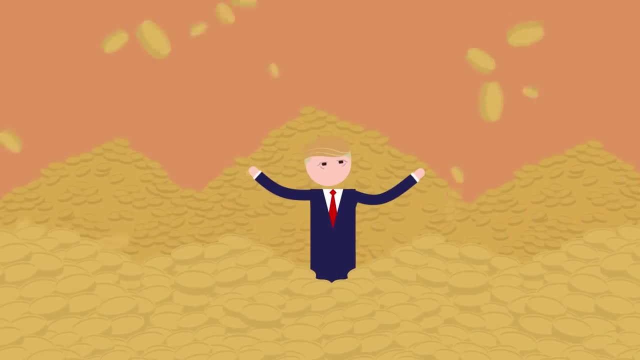 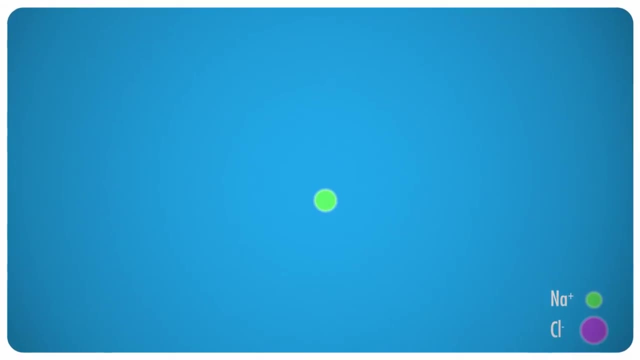 The electron is to chemistry what money is to capitalism. It's all about who has it, who wants it and what they're willing to do to get it. Electrons are what make it possible for an atom to bond with other atoms, to form molecules. 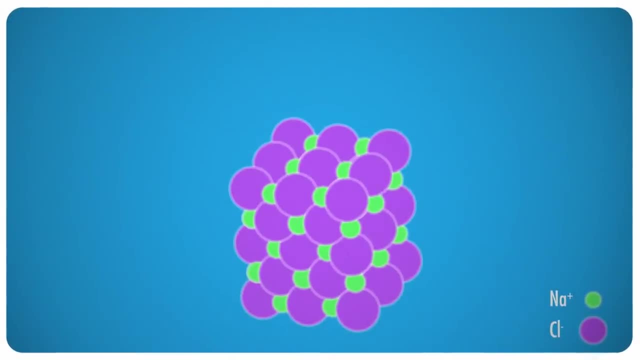 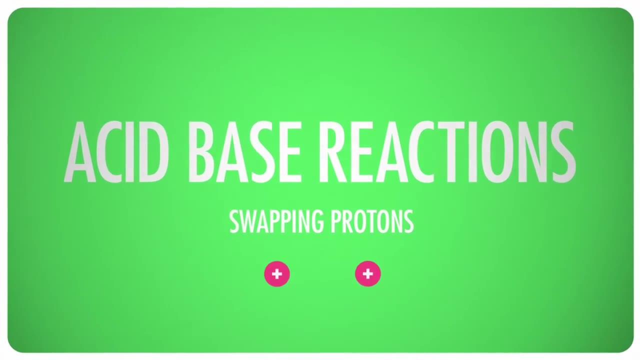 and when that happens, a tremendous amount of energy can be exchanged in the process. But not all chemical reactions involve electrons changing hands. Acid-base reactions, you'll recall, are more about swapping protons, But because electrons are the real coin of the 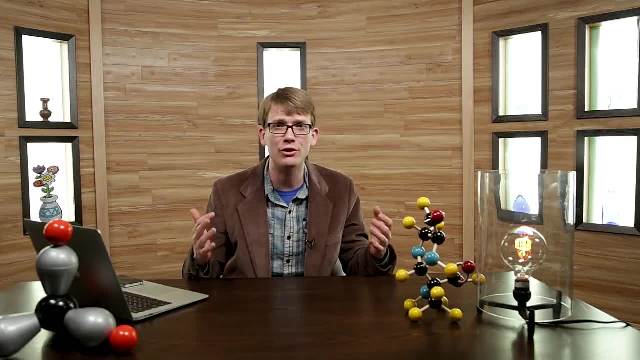 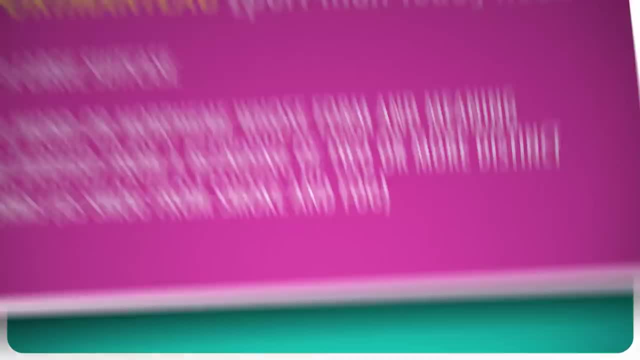 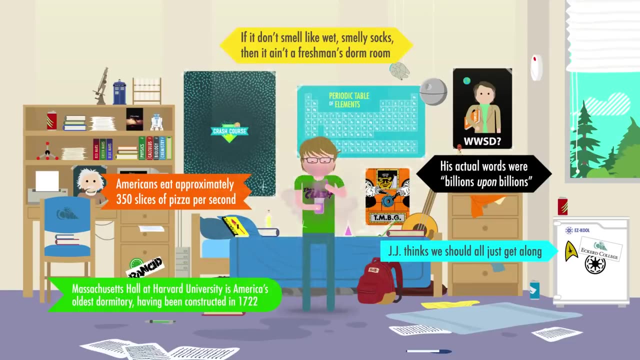 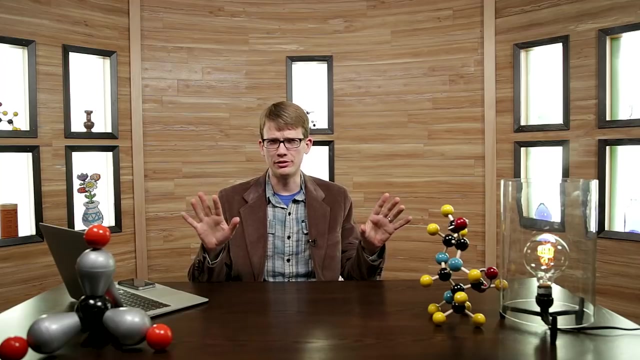 realm. in chemistry, the most important reactions that take place on Earth involve the transfer of one or more electrons from one atom to another. These are redox reactions, Redox, which is a portmanteau of reduction, oxidation, But what's up with those words? You know what reduction is: Making less of something, And 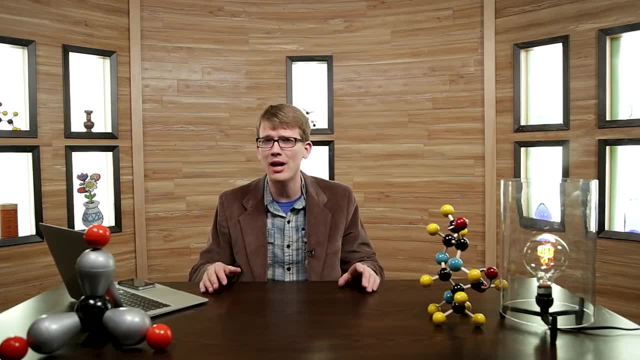 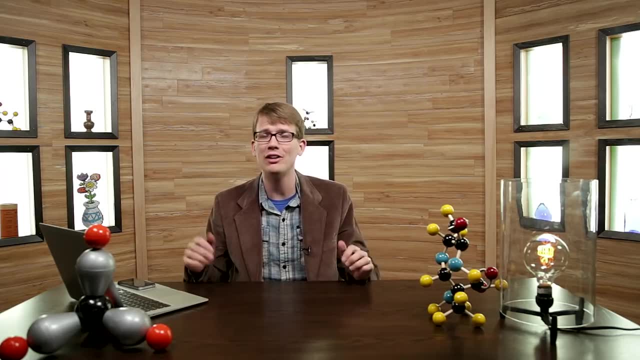 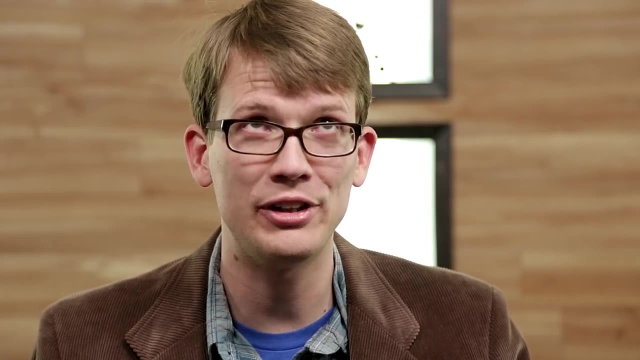 then oxidation maybe has something to do with oxygen. Well, sometimes, but not always, These are actually super-efficient reactions. There were terrible choices for what is actually happening in redox reactions, but we are stuck with them. Reduction is when a substance gains electrons. Yes, it gains, which is the opposite of what. 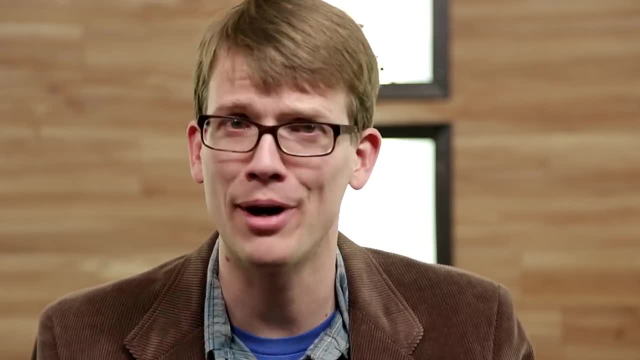 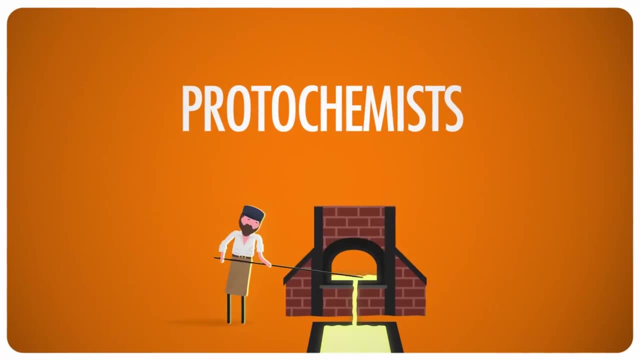 the word produce means Fantastic, And, yes, sometimes I want to punish the people who named these things so inaccurately, but they didn't know any better and they're all dead, so we can't do anything about it. Protochemists would make pure metals by heating or smelting their ores, And they noticed. 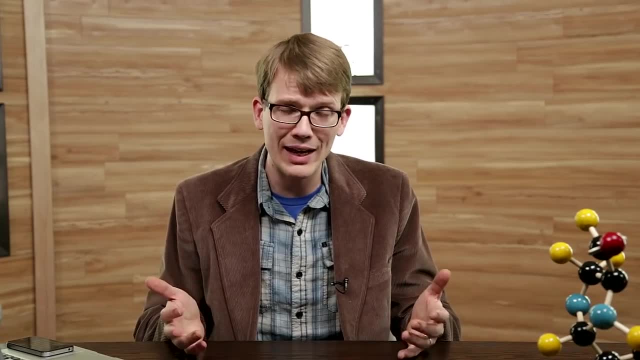 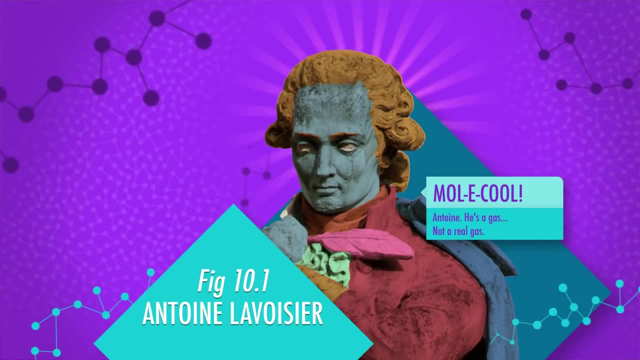 during the smelting that these substances would become lighter. So I guess they were right. So I guess it's not crazy that they decided to say that these substances were being reduced. Our old French friend, Antoine Lavoisier, figured out that this was because oxygen gas was actually 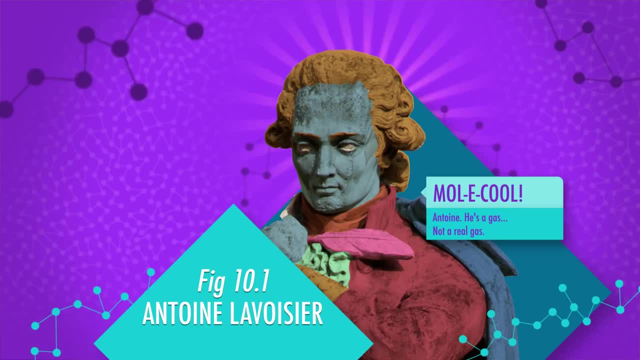 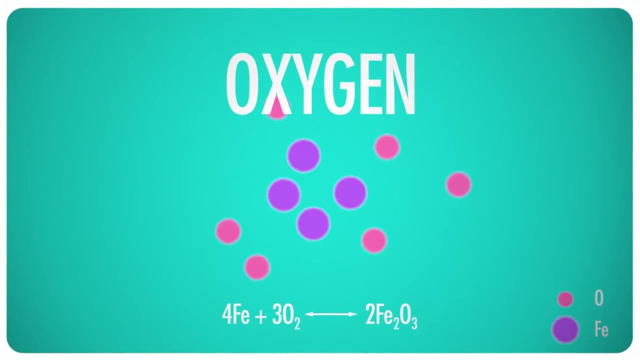 leaving the compound, making it lighter. What he didn't know was the actual chemistry involved. Oxygen is, unsurprisingly, the quintessential oxidizer. It pulls electrons off of one molecule to make itself more stable, But if you heat it up enough, it gets all energetic. Today, 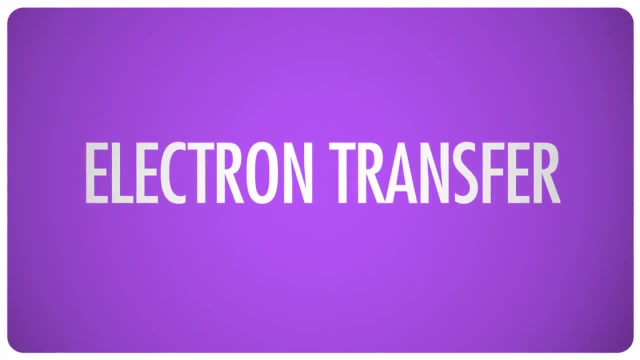 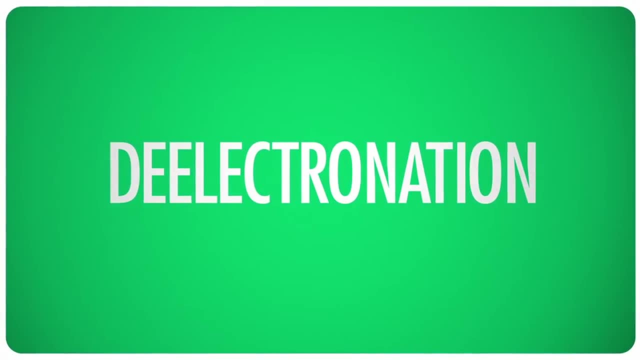 we understand that oxidation and reduction are all about electron transfer, So you might think that we'd rename them, And some chemists have tried producing terms like electronation and deelectronation. But once a set of terms is decided upon and used for, 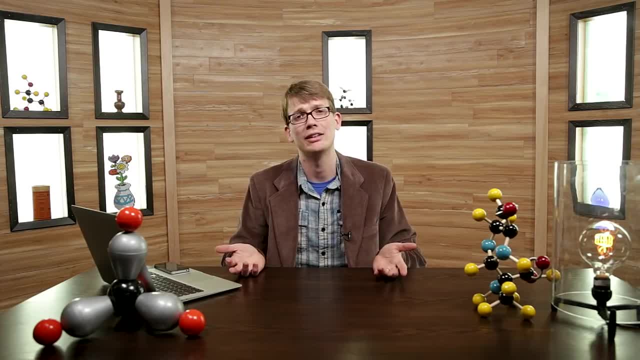 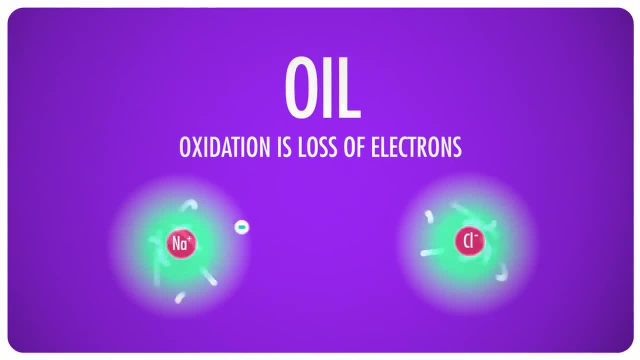 a while. it's pretty difficult to uncreate it, So we're stuck To keep these seemingly nonsensical names straight. I rely on the phrase oil rig. Oxidation is loss of electrons, Reduction is gain of electrons. We just gotta know this stuff. 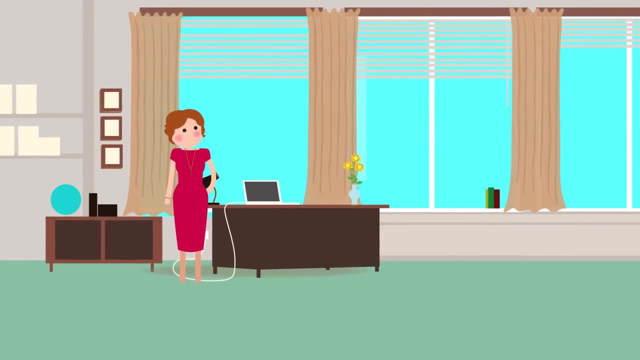 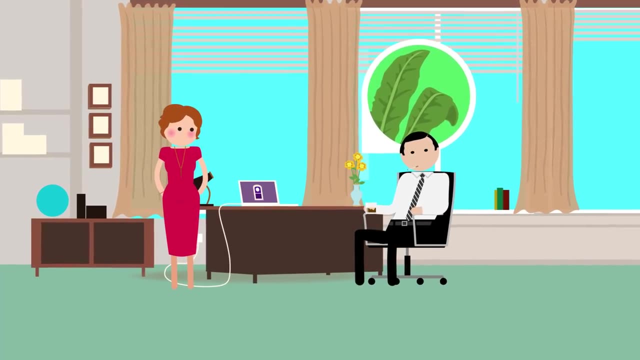 because it's everywhere. When your cells convert sugar into energy so you can move and breathe and think, that's redox. When plants photosynthesize sunlight into food, that's redox. The battery powering your laptop: Redox. Fire, Also redox, Since electron swapping is the name of the 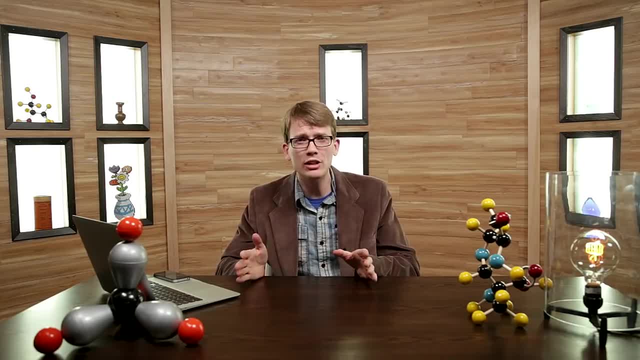 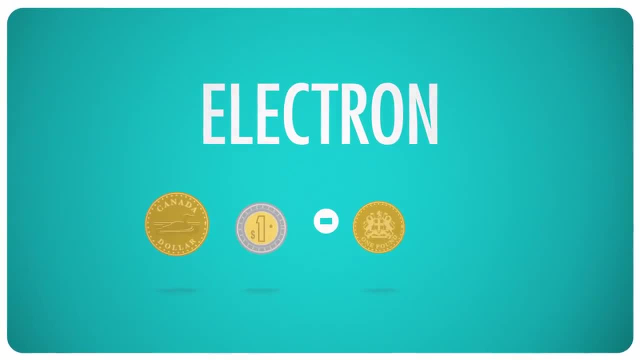 game here. when you study redox reactions, it's important, critical, absolutely essential to keep track of the electrons. Think of them as dollars or pesos, or pounds or euros. In any transaction, one person is going to gain them and the other is going to lose them. 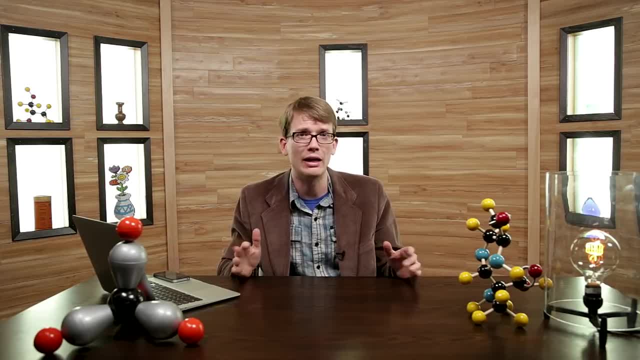 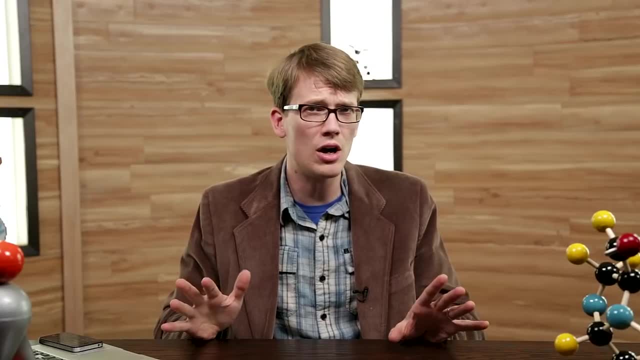 And to stay on top of things, you have to keep tabs on who's ahead and who's behind. Atoms are fond of sharing electrons though forming covalent bonds, so sometimes keeping track of where they are and where they're gonna end up isn't quite so simple. 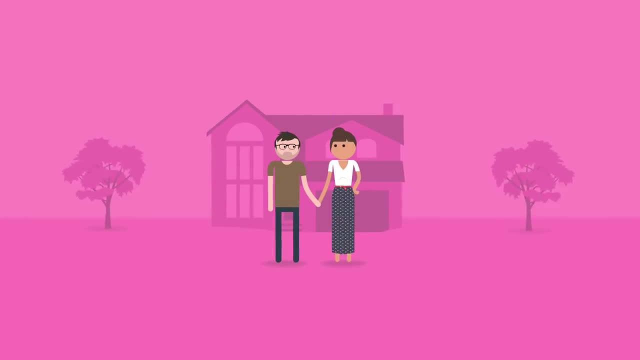 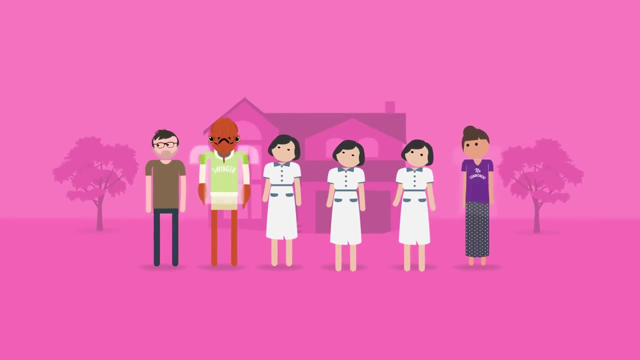 Let's think of every covalent compound like a marriage, though it's gonna be a weird marriage because, like there might be like six people in it, sometimes the same person several times without commitment. no commitment and also no emotions. Don't think too much about it. Like in a marriage where money gets shared, covalent compounds share electrons, The trick is figuring out who gets the cash when the vows break. So we've created a useful little system assigning electrons 100% to atoms that are actually. 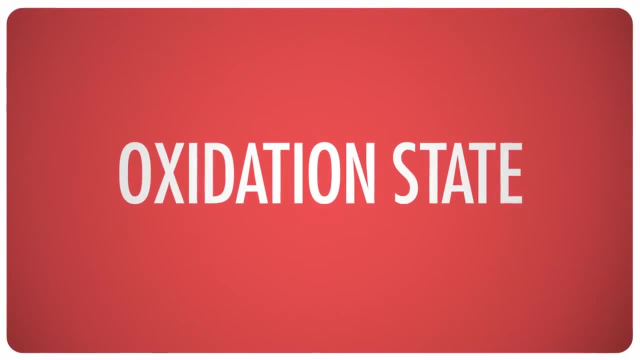 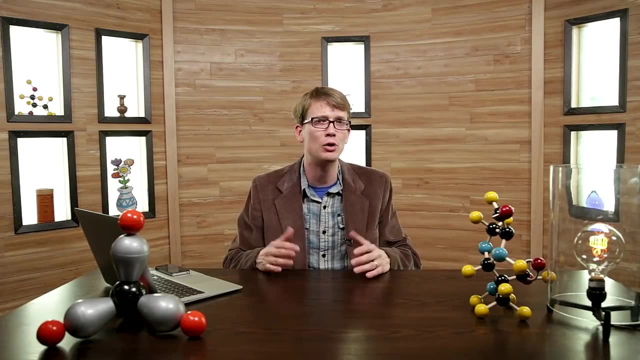 at the moment sharing them. The number that we assign is the atom's oxidation state or oxidation number, Even though we are, of course, aware of covalent bonds and the sharing of electrons. the processes are easier to follow if we imagine that the atoms are already splitting up. the bank account as if they were in an ionic or nonsharing bond. So when atoms oxidize, this hose will get back up. but I say this oxidation number is basically what its charge would be if it actually owned all of its electrons. 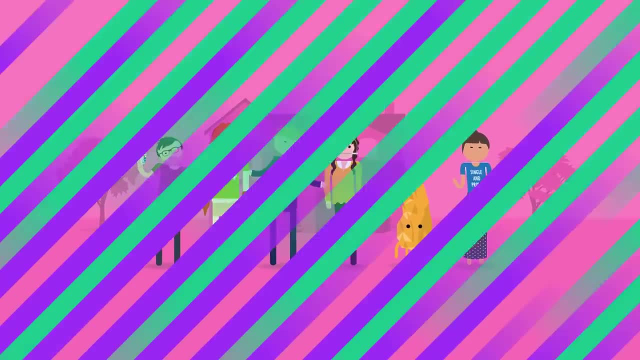 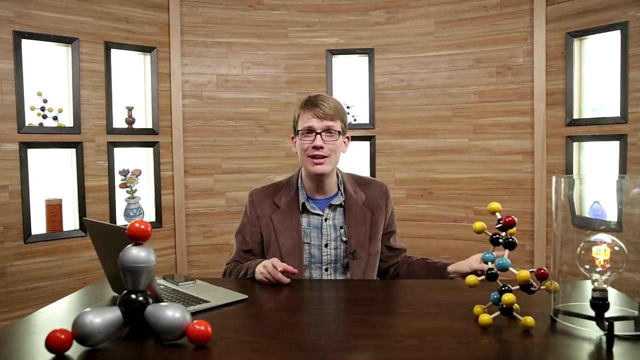 exclusively like the newly minted bachelors that they may become. So to figure out those oxidation states or oxidation numbers, we have some simple rules for some atoms. First, the oxidation number for any element by itself, whether it's monatomic. 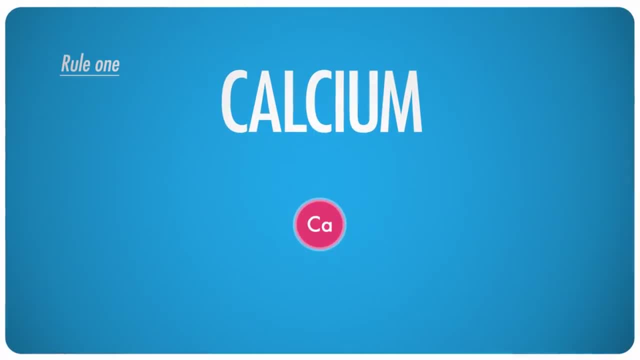 or diatomic or polyatomic, like an atom of calcium or a molecule of H2, or an even bigger molecule of sulfur, S8,. the oxidation number is zero. Atoms, by definition, do not have a charge. If they had a charge, they would be ions, and if they're sharing with themselves. 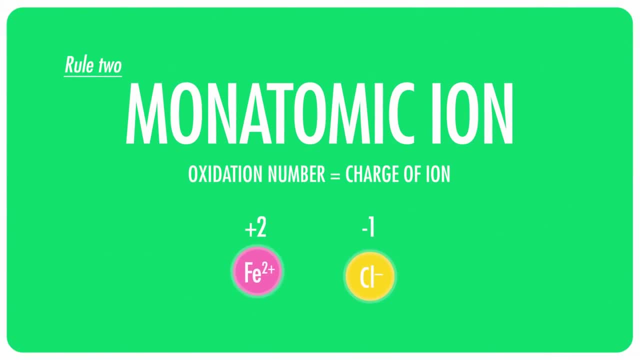 they share equally. Second, for a monatomic ion, basically a charged atom, it's simply the size or number of its charge. So the iron two in Fe2 plus has an oxidation state of plus two, while a chloride ion is minus one. Third, oxygen, which is unsurprisingly all. 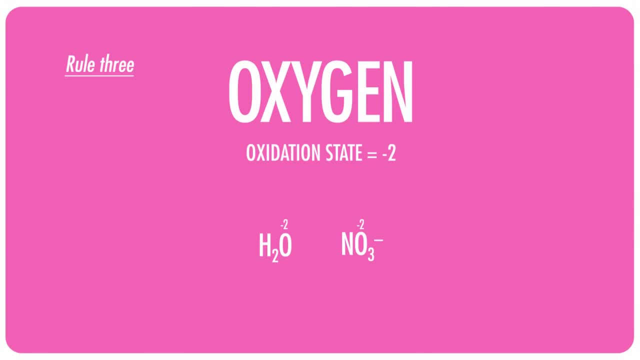 over redox. chemistry almost always has an oxidation of negative two, unless it happens to be in a peroxide molecule like hydrogen peroxide. Fourth, hydrogen is plus one and fifth, Fluorine is negative one, as are all the other halogens most of the time, Pretty much. 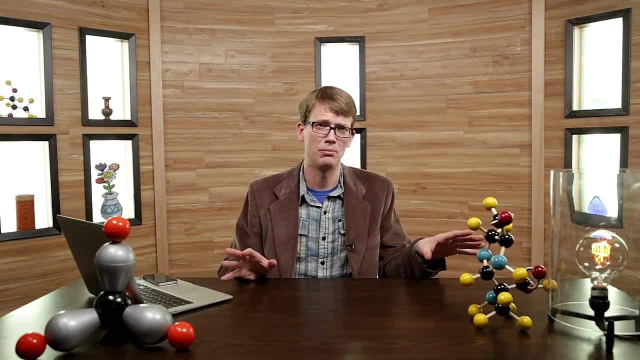 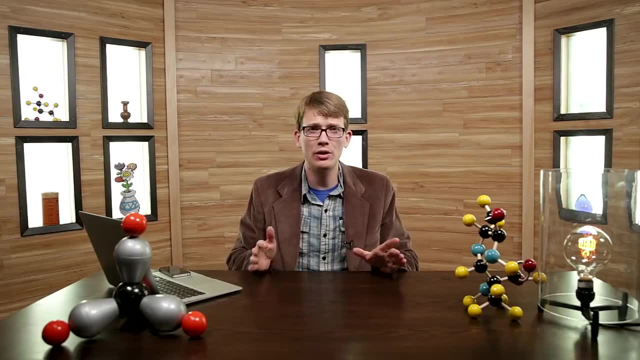 unless they're bonded to fluorine or oxygen, because fluorine and oxygen are so bad that they can make anybody's oxidation number positive. if you know what I mean, And those are the rules, That's all you need to know. Now, the total of all the oxidation numbers of all 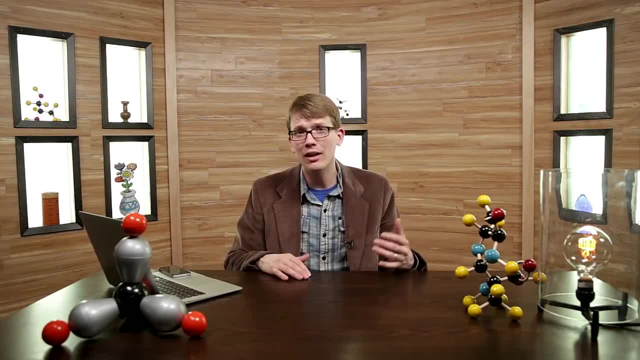 the atoms in a neutral compound will add up to zero, Like water, with one oxygen with a negative two oxidation state and two hydrogens at plus one. and voila, the neutral compound has an oxidation number. A polyatomic ion, on the other hand, has to work out to have an oxidation state that 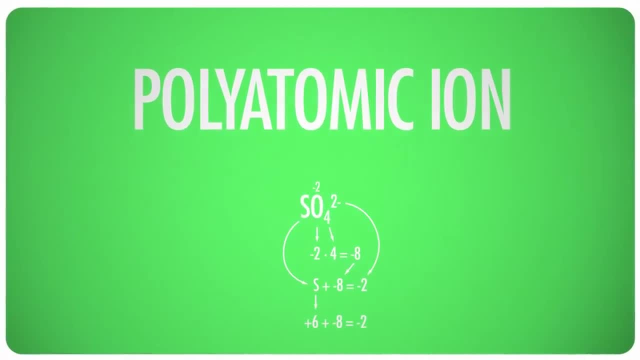 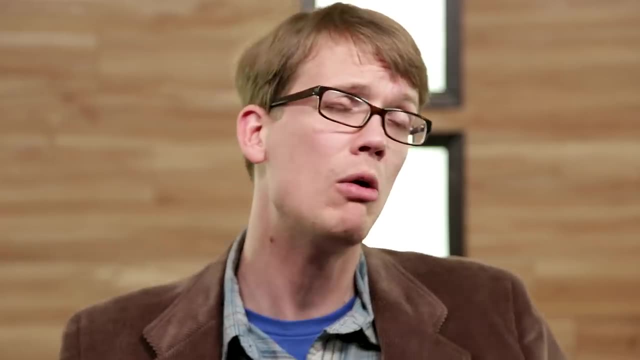 matches its charge. So SO2-, the sulfate ion, has four oxygens for a total of negative eight. but we don't have a rule for sulfur, so I guess we just give up and walk away. Who cares anymore? No, We used like third-grade algebra, because we have to end up with an oxidation number. 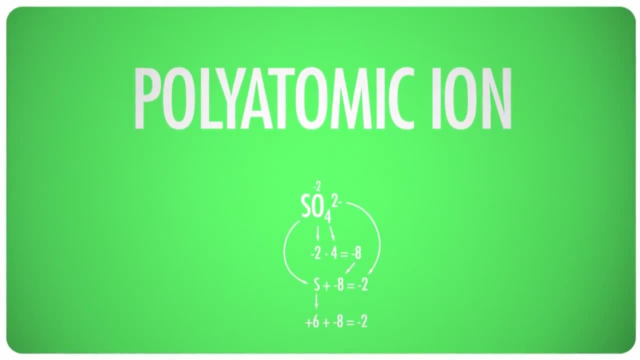 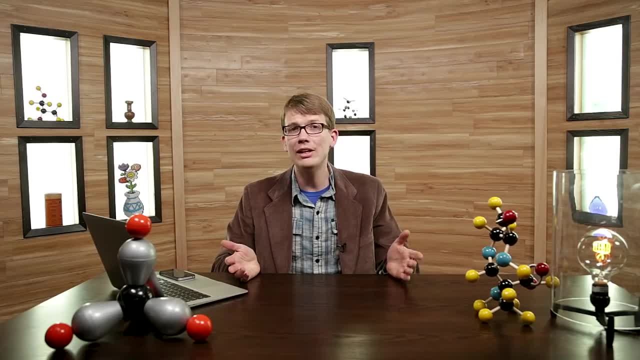 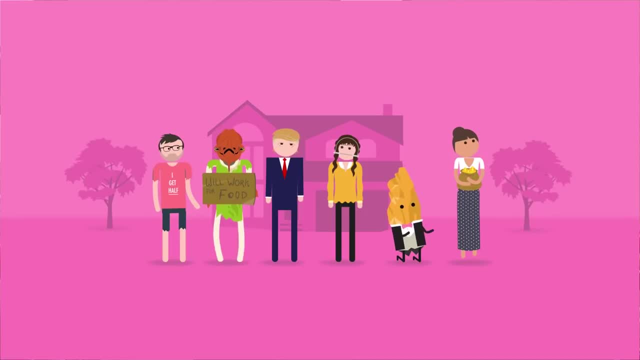 states of most elements change depending on what they're bonded with. Now we can use this same logic to figure out what happens when these compounds interact in redox reactions: Molecular divorce, courts of electrons changing hands, being haggled over and treated, with some players taking big profits while others lose nearly everything. 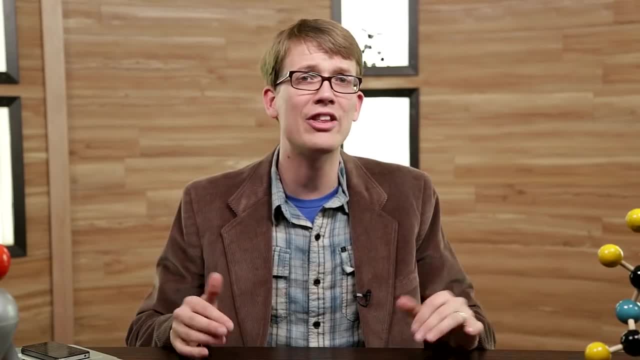 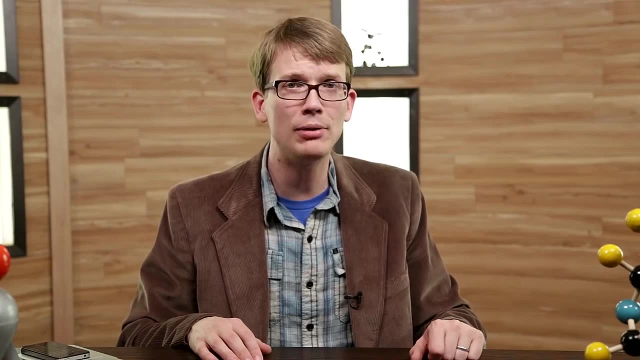 Them's the breaks. Let's start out with a simple example, a chemical reaction that I believe has saved more lives than any other in the world In the history of chemistry: created by a war criminal to blow people up during World War I: the Haber Process. 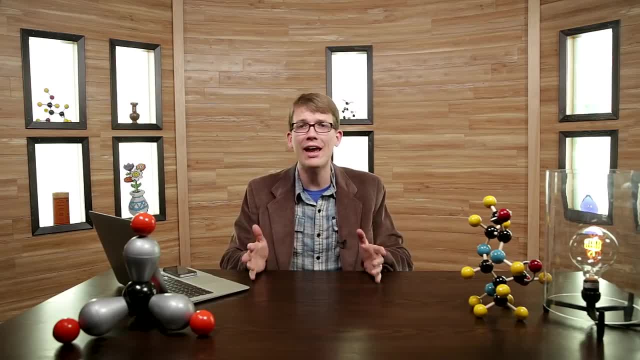 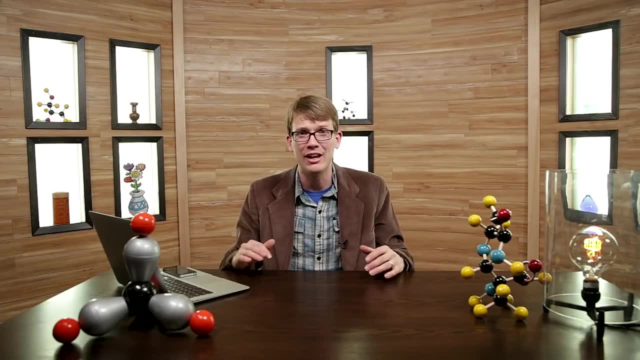 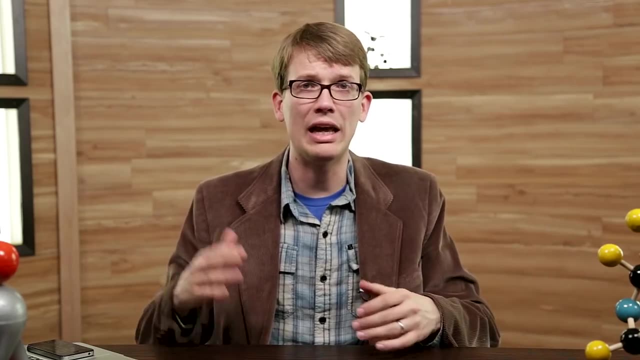 The Haber Process removes the ultra-stable elemental nitrogen from the air and combines it with hydrogen to form NH3, ammonia, for use in bombs and also in fertilizer, increasing the carrying capacity of the earth by billions. Nitrogen in the air exists as elemental diatomic nitrogen, and hydrogen likewise as also diatomic. 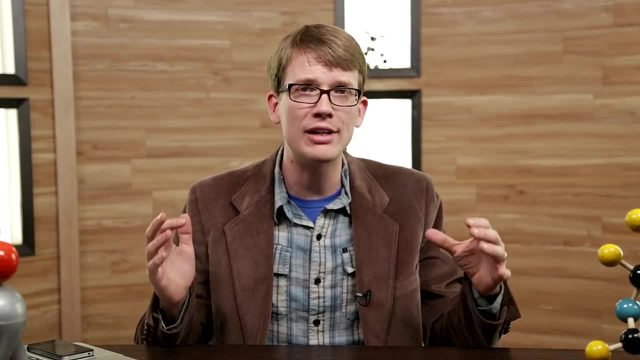 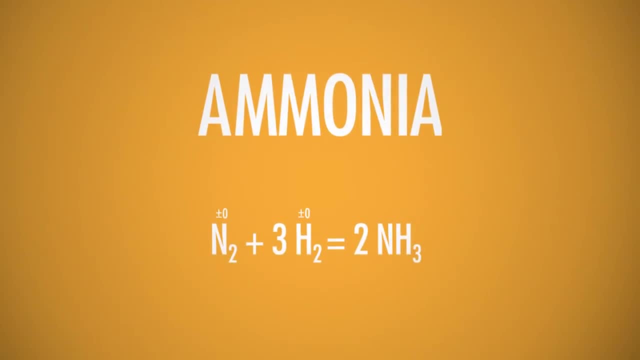 H2.. So we know that, starting out, all of the atoms have an oxidation state of zero. The product of the reaction, ammonia, is a neutral compound with one nitrogen and three hydrogens. The hydrogens each have an oxidation state of plus one. remember the rules. so 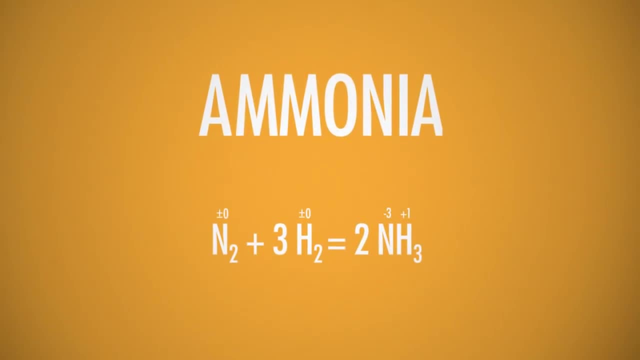 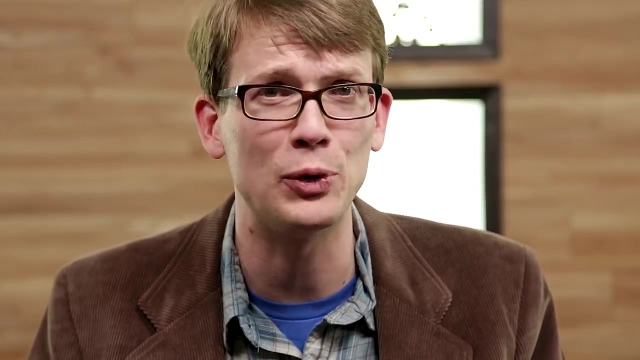 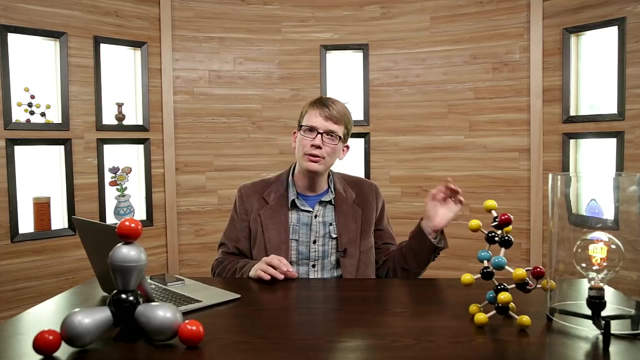 nitrogen must have an oxidation state of minus three. Nitrogen thus gained electrons. its oxidation state went down, and so it was reduced. So at least when talking about what oxidation states are doing, the word reduced makes sense. Hydrogen lost electrons. the oxidation state went up and it was oxidized. Now this is. 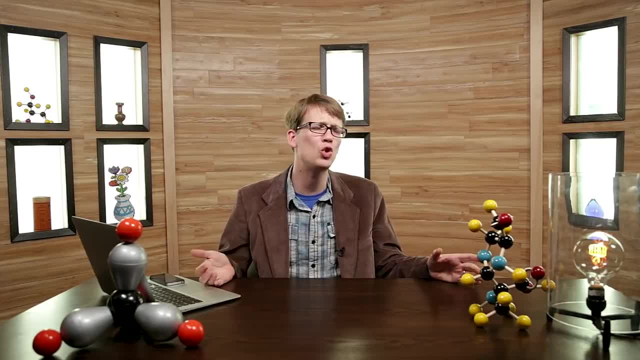 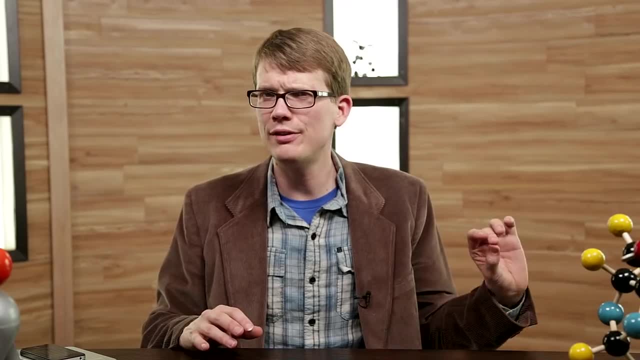 a pretty simple equation to balance, But redox equations can be a huge headache sometimes because of the number of individual atoms involved, so we often have to balance them in half reactions. So, even though we don't really need to do the half reactions, because this is a pretty 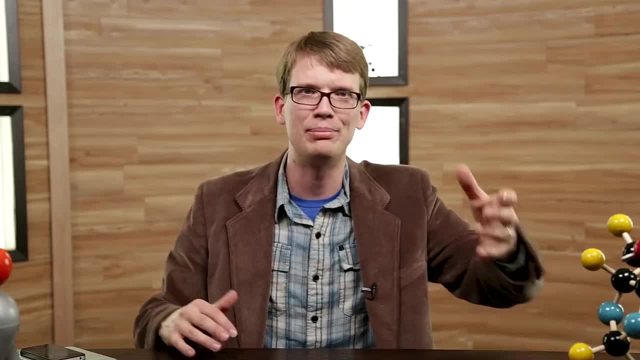 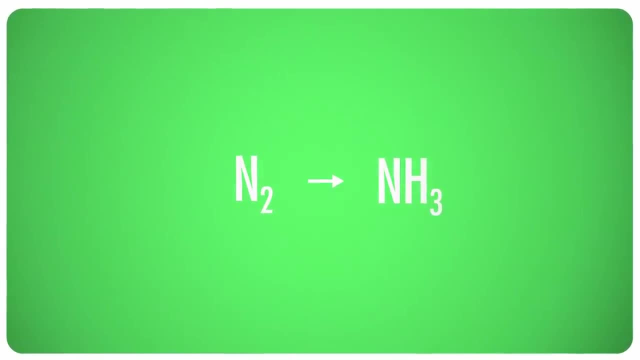 simple equation. we're gonna do them anyway, just because it's an example. that's simple to start with. So start out, with the nitrogen getting reduced, We have N2 with an oxidation state of zero becoming NH3 with an oxidation state of negative three. 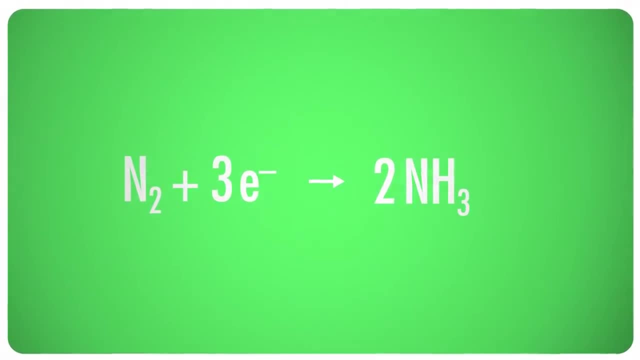 First we balance the number of nitrogens, then add the number of electrons that we need to have to have there be the same number of electrons on each side. Do the same with the oxidation half of the reaction and then combine them to get your 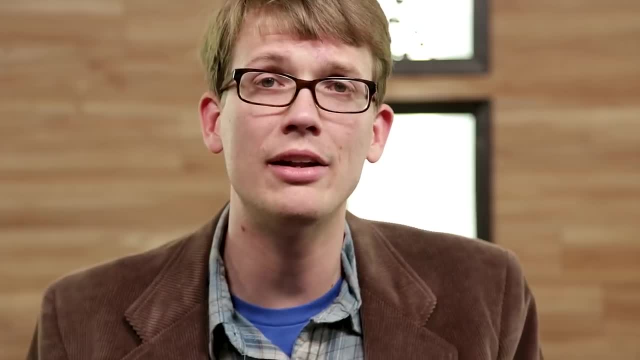 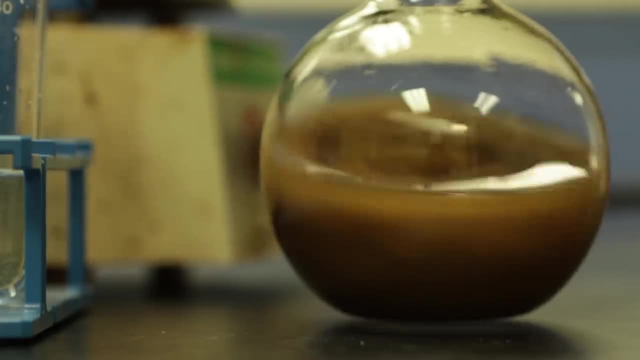 whole reaction with the electrons cancelling out. Now, yes, maybe that seemed like an unnecessary step, but allow me to show you a more complicated example that will prove how necessary it may be. In this flask is silver diamine. We're going to use some redox chemistry to get the elemental 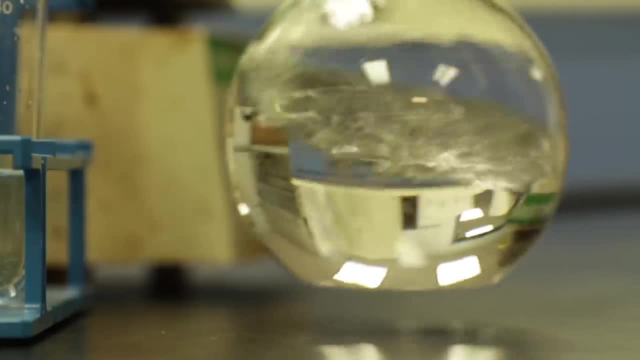 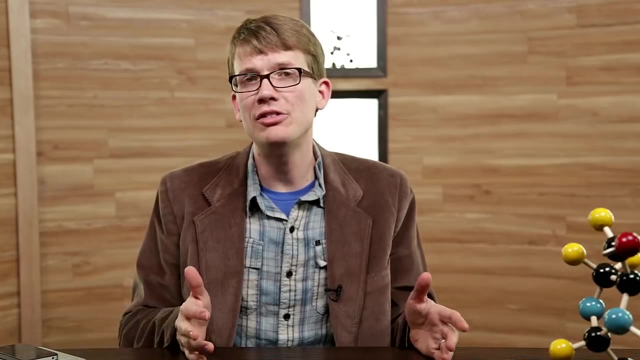 silver out of it nice and clean and shiny, and it's not gonna be no simple Haber process. The silver diamine is going to react with an organic aldehyde, Any aldehyde, And it's any aldehyde. actually, The business end of the aldehyde is the CHO end. The R in organic chemistry is a symbol. 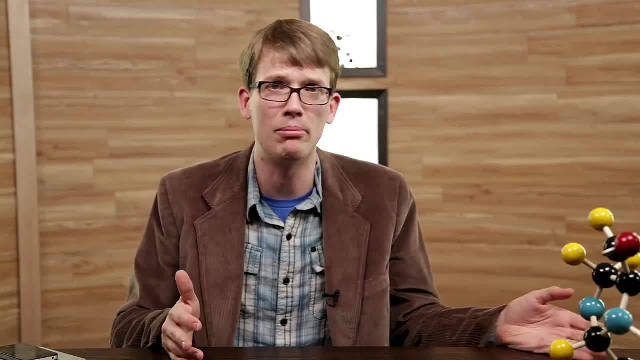 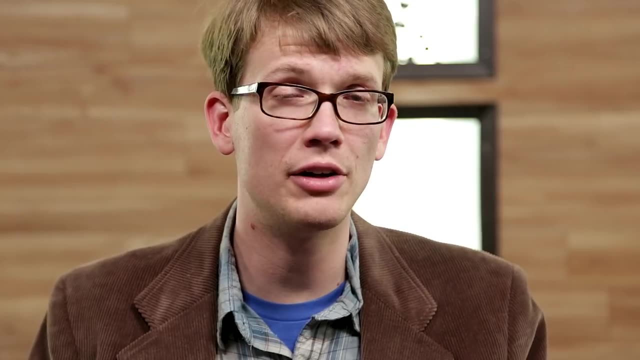 for some organic group of atoms, and in this reaction those atoms don't matter. The silver diamine reacts with the aldehyde and hydroxide, creating carboxylic acid, ammonia and water. First let's assign ourselves some oxidation states. 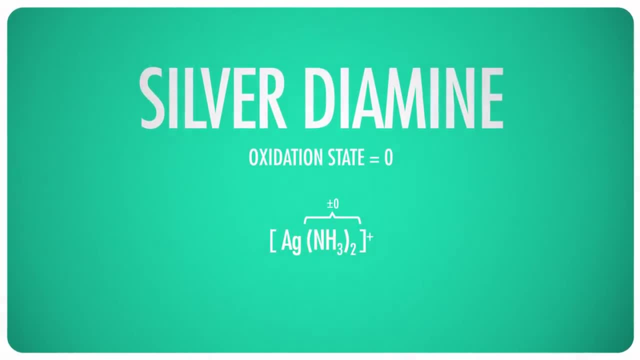 The silver is in a complex with two neutral ammonias that are going to remain unreacted throughout the equation, so we can treat them like a single species with an oxidation state of zero, Since the silver diamine has a charge of plus one and the ammonias don't affect that. 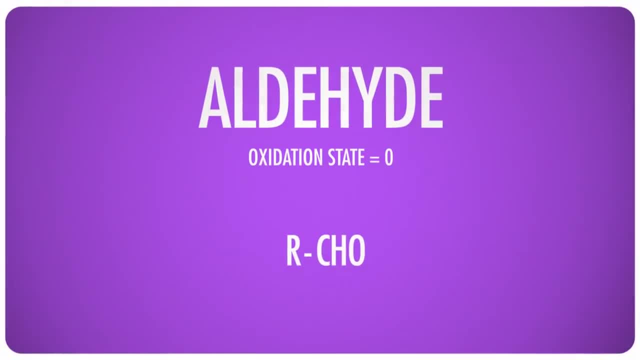 silver's oxidation state must also be plus one. The aldehyde has one hydrogen at plus one and one oxygen at minus two, but is neutral overall, so the carbon must be plus one as well. The hydroxide ion is simple: minus two for the oxygen, plus one for the hydrogen, and 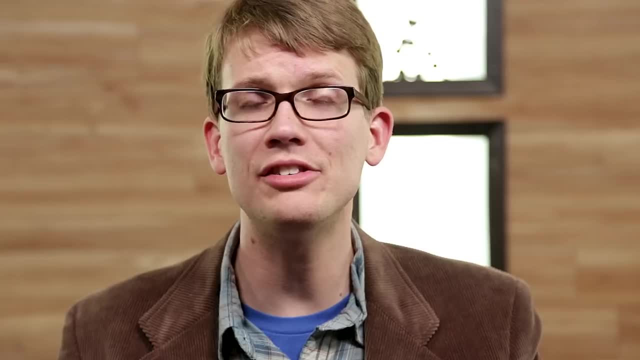 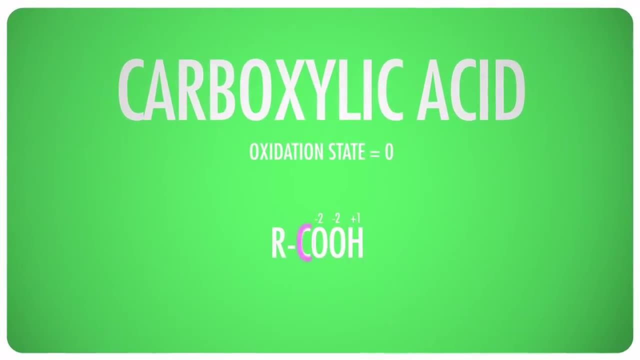 an overall charge and thus oxidation state of minus one. On the reactant side, the silver is now atomic, so its oxidation state is zero. The carboxylic acid has two oxygens And one hydrogen, so the carbon now has an oxidation state of plus three. NH3 remains. 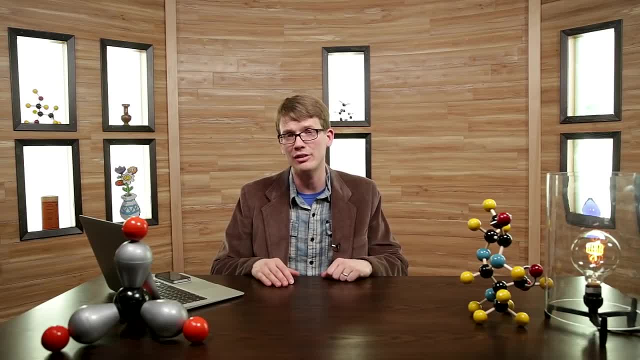 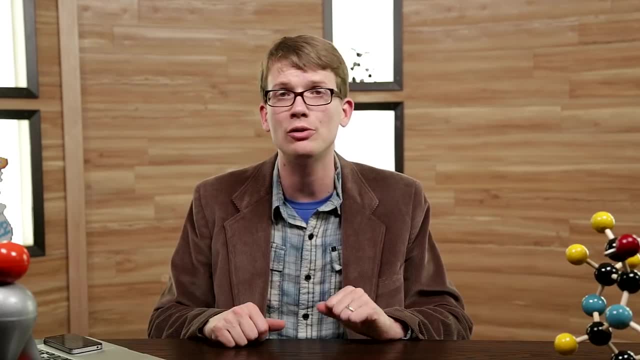 at zero, and the hydrogen and oxygen of water also haven't changed oxidation states. So silver's oxidation state decreased or was reduced from plus one to zero, while carbon was oxidized from plus one to plus three. Half-reaction time: 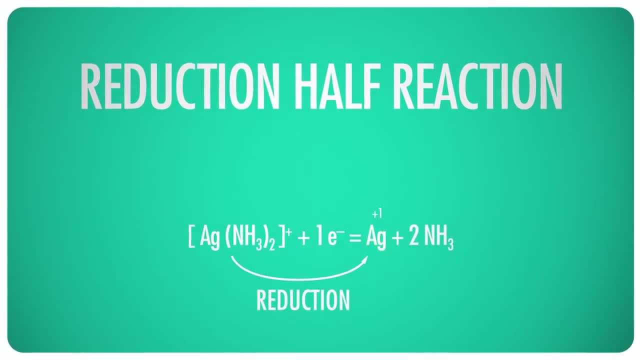 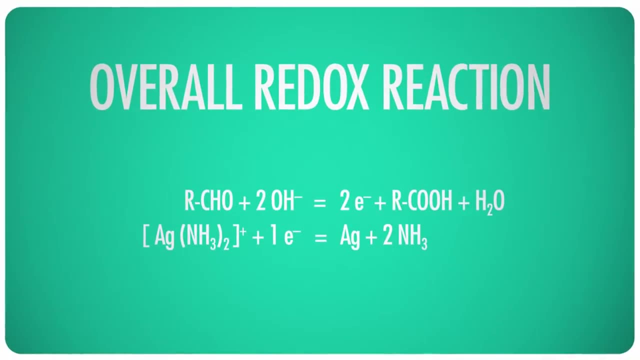 Silver was reduced, gaining one electron forming elemental silver and ammonia. from silver diamine, The aldehyde was oxidized, forming carboxylic acid and requiring two electrons. With the help of those electrons, we know that at the end of the day, we're going. 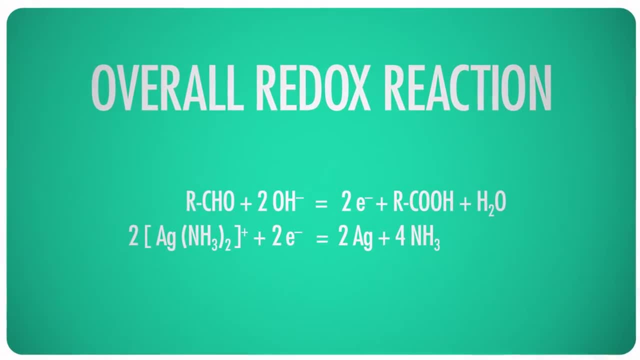 to have two electrons, But at the very least we have to double the reduction half of the equation entirely in order to get the right number of electrons on both sides. We do that- and oh god, that's good stuff- And we combine them together for a perfectly balanced redox equation. 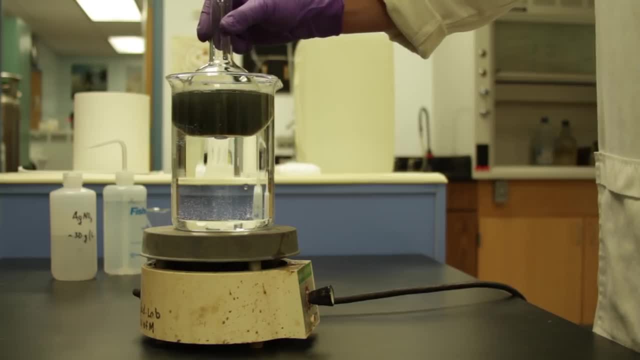 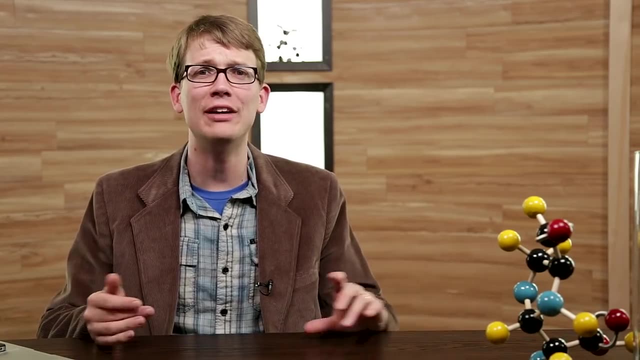 And now watch me dig those electrons and turn them into money. And there you have it. folks, That is pure silver coating the inside of the flask. Thank you for watching this episode of Crash Course Chemistry. If you were paying attention, you learned that any reaction where electrons move around, from atom to atom is a real reaction, And that's why you're watching this episode of Crash Course Chemistry. If you were paying attention, you learned that any reaction where electrons move around from atom to atom is a real reaction, And that's why you're watching this episode of Crash Course Chemistry. If you were paying attention, you learned that any reaction where electrons move from atom to atom is a real reaction. 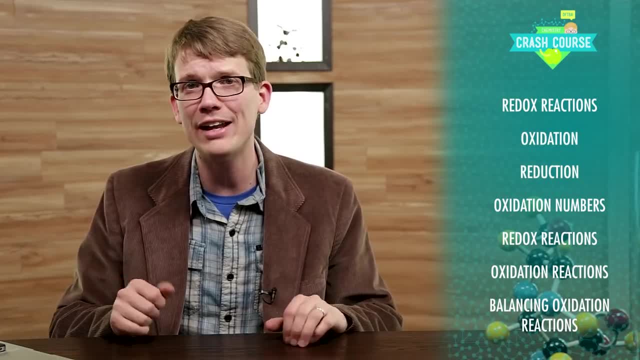 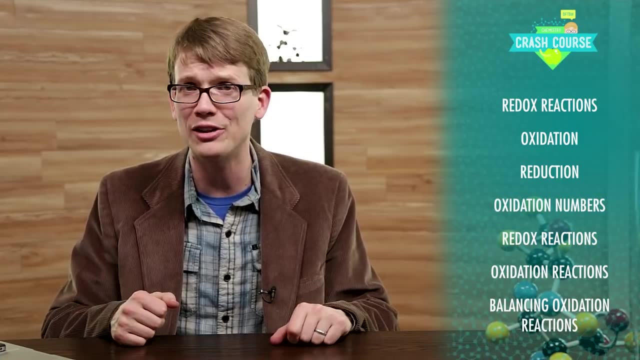 That oxidation is the laws of electrons and that reduction is the gain of electrons, And that oxidation numbers are assigned to atoms to take part in reactions in order to keep track of what their electrons are up to. You also learned a few simple tricks to help figure out what an atom's oxidation state.